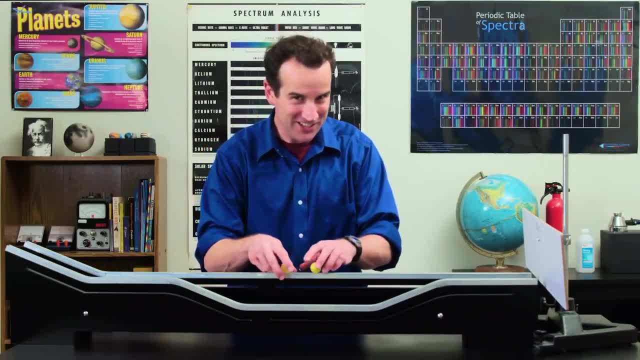 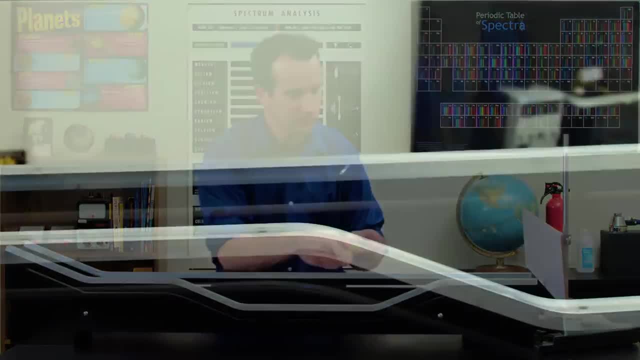 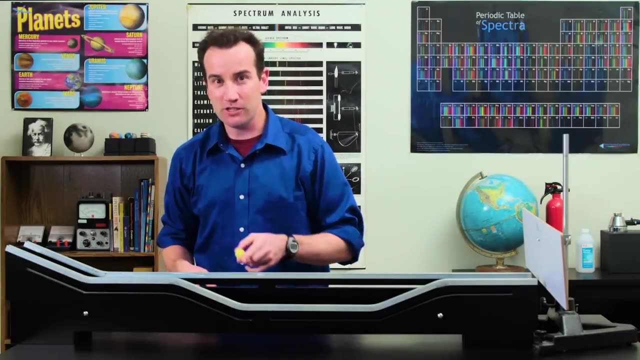 One of the best energy demos is this racing marbles lap. Two marbles are released from the same height and race along different paths, But which one will reach the finish first? Make your guess and tell the person next to you why you think you're right. 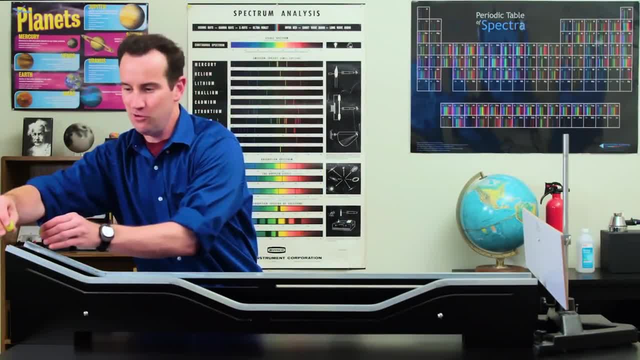 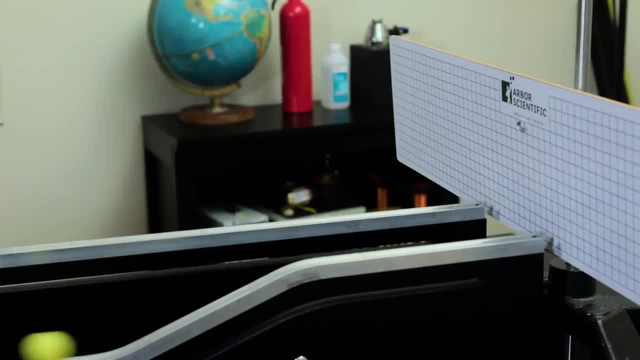 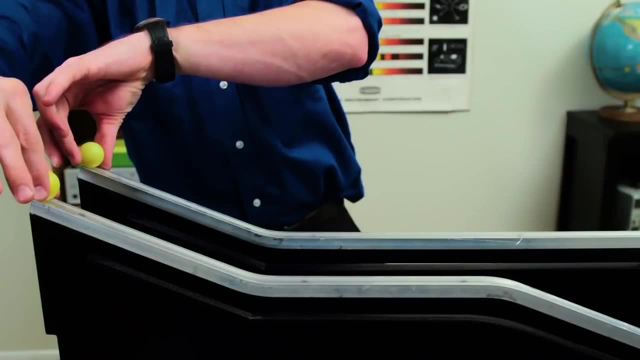 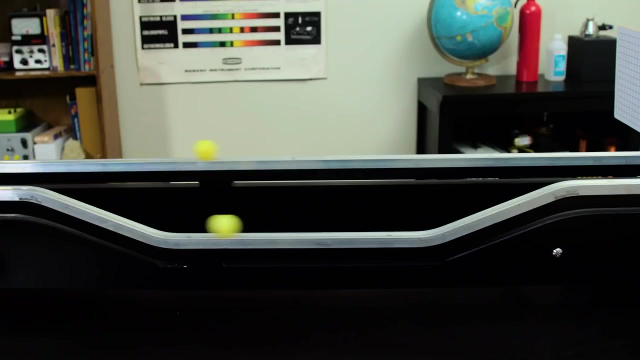 Alright, here we go: Three, two, one. Now that you have seen the result, explain it correctly. The marble that was allowed to dip lower got to convert its potential energy into kinetic energy, which let it go faster. The higher marble moved at pretty much the same constant speed. 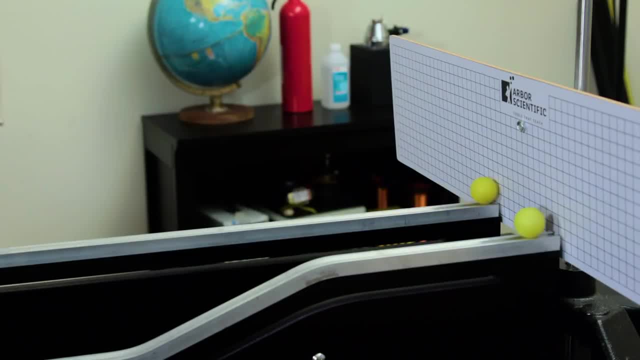 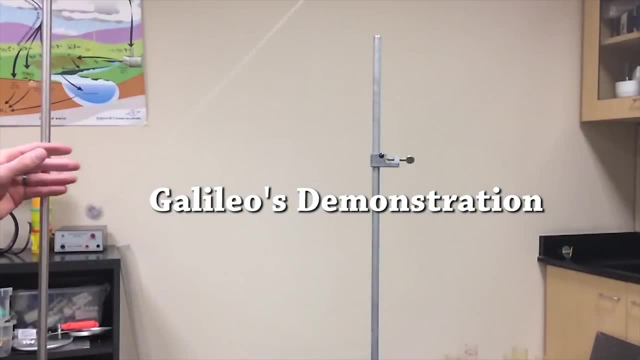 By the end of the race. they do both finish at the same speed, just not at the same time. We can introduce the idea of energy the way Galileo described it: A pendulum is swung from a specific height And somehow it always seems to remember the height from which it was released. 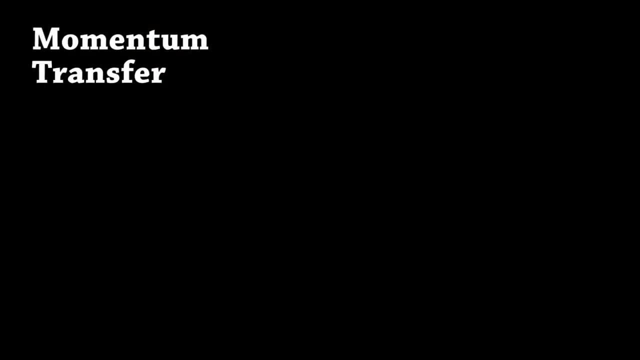 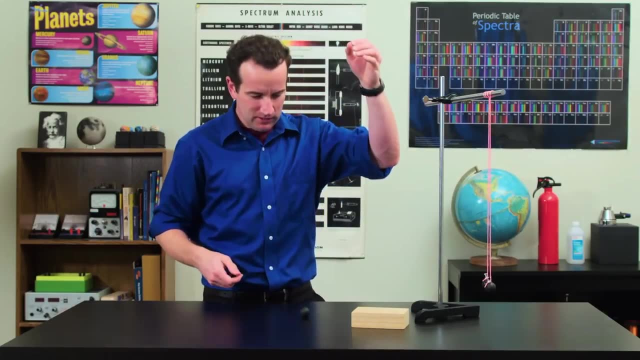 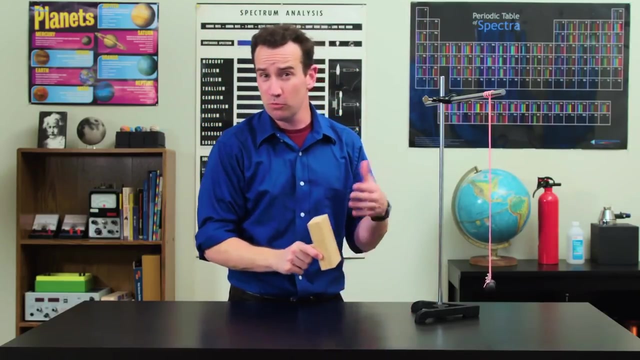 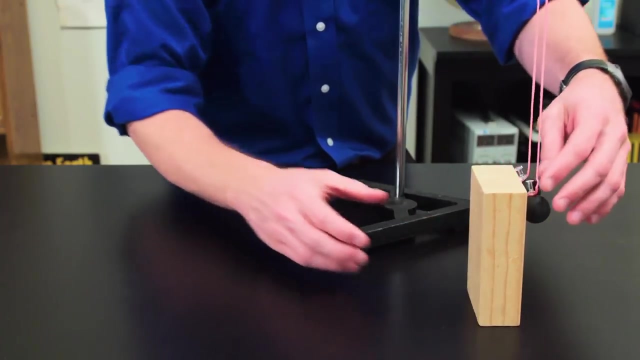 How does it remember? Momentum is transferred by collisions? This ball does not bounce, But this ball bounces. well, Which of these two is more likely to knock over the wood block? Make your guess First. we test. the doesn't bounce. 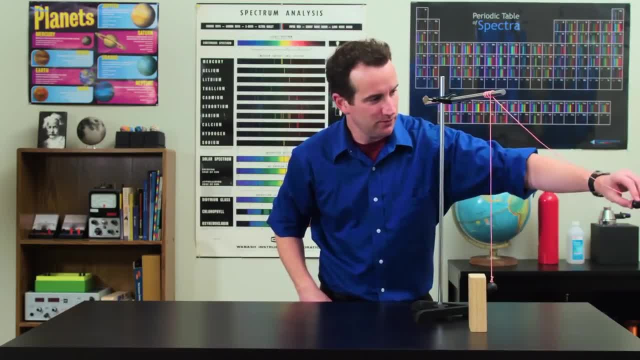 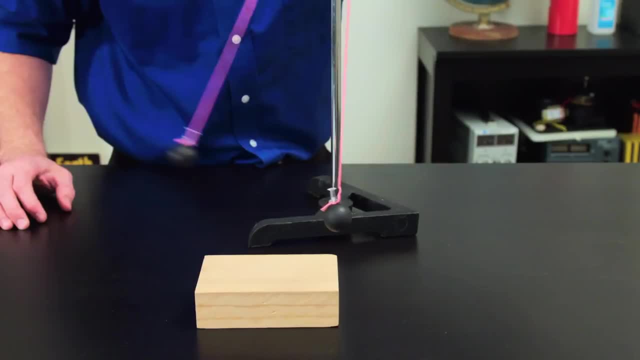 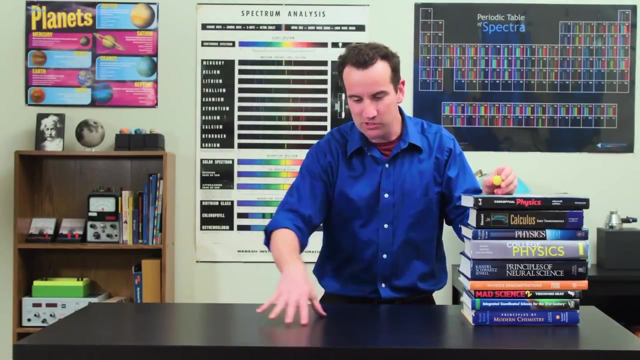 Doesn't work. Now the bouncy ball. Huh, The bouncing transfers more momentum because it bounces backwards with negative momentum. The total change is larger than just coming to a stop. Most people understand that potential energy is relative to some zero-energy point. 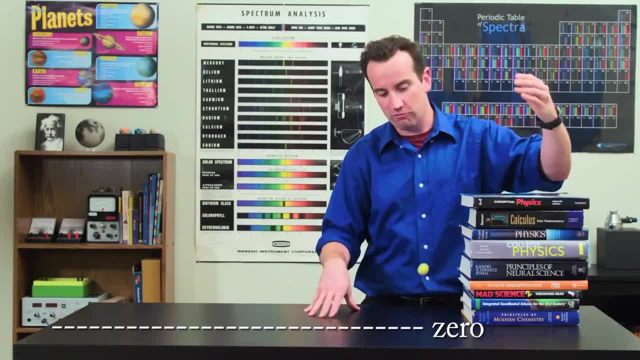 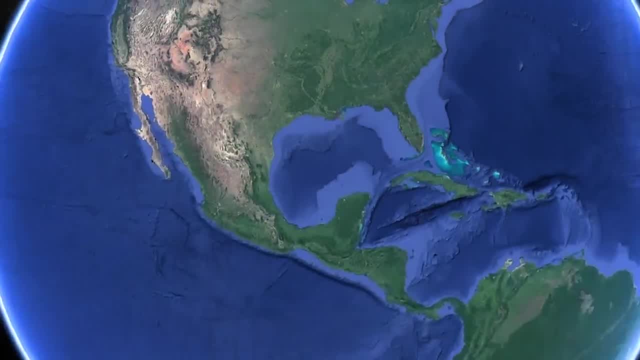 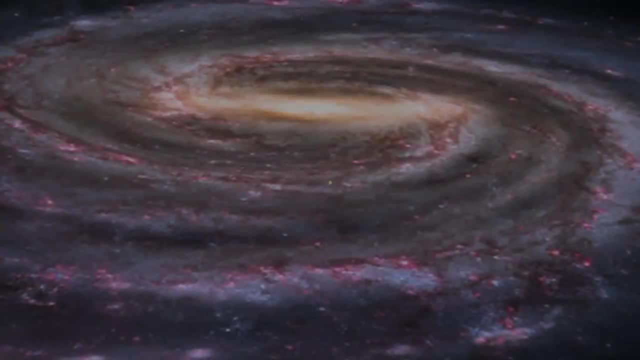 For example, this ball has the potential to roll off a stack of books to the table, but it could also fall off the table to the floor And it could even fall down a well to the center of the Earth, And it even could fall to the center of the Milky Way galaxy. 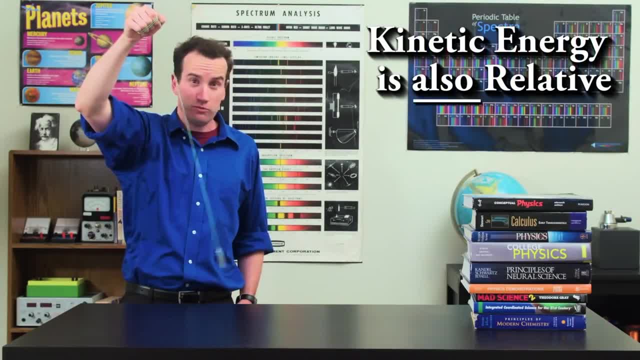 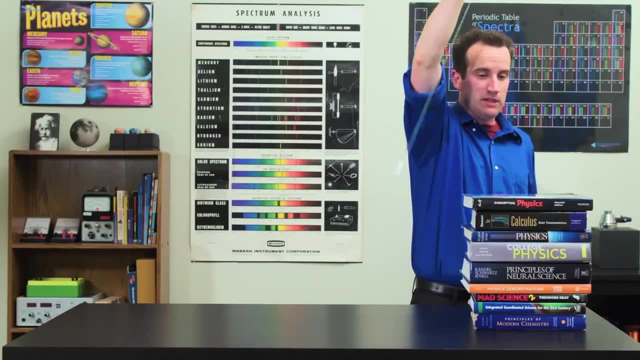 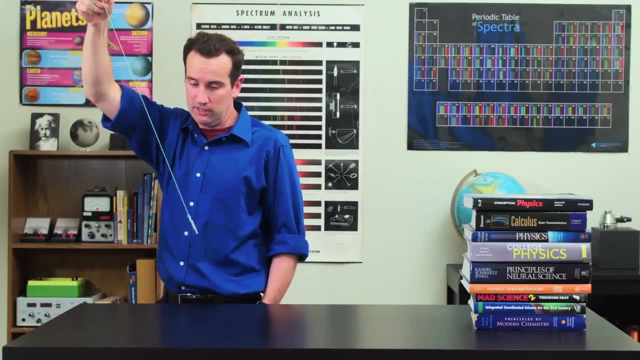 But how do I demonstrate that kinetic energy is also relative? Well, if I walk with this pendulum, I show that its motion is relative to me. In fact, my calculation of its kinetic energy depends on how fast I'm moving. If we move together, I might calculate that it has no kinetic energy. 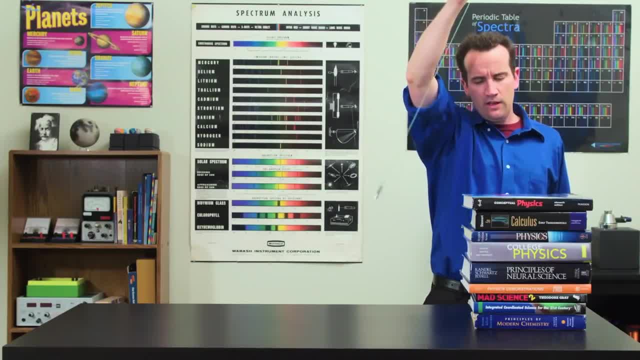 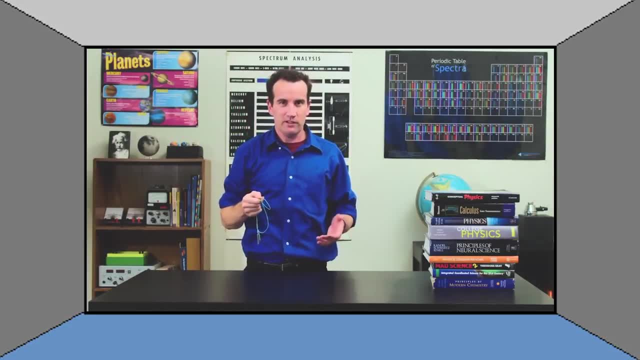 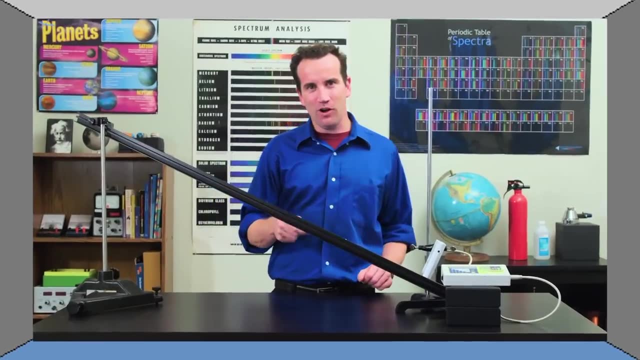 until I stop and it looks to be swinging again. Normally, we use the laboratory frame as a method to calculate the relative velocities, For example. this would be zero and anything else would be non-zero. At the beginning of the video, I promised to show you that energy and momentum were not the same thing. 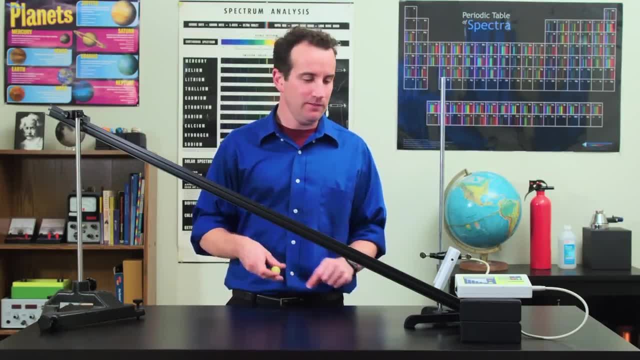 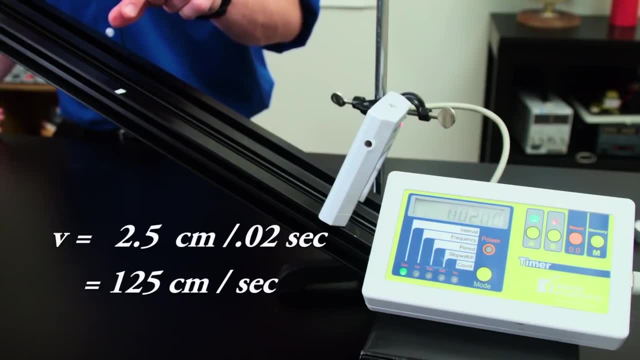 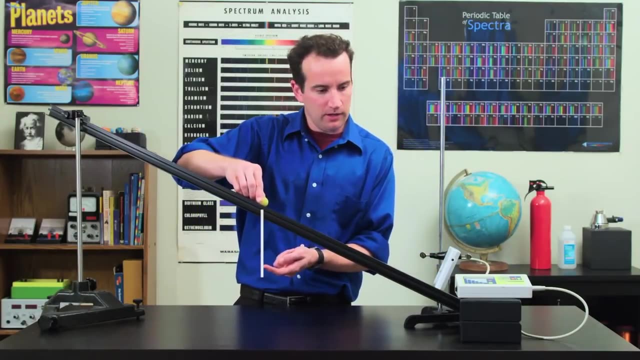 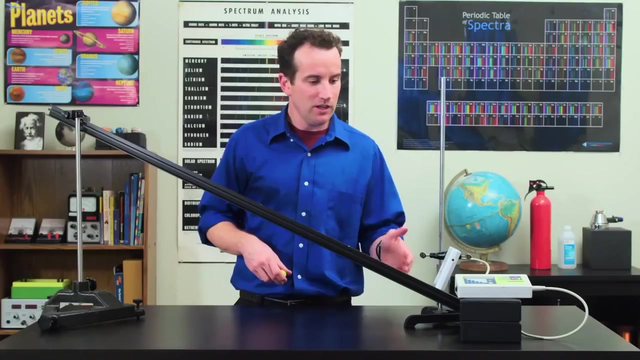 And this lab proves it immediately. If I let the marble roll from 10 centimeters up, I get this velocity. If I repeat the experiment from 20 centimeters up, I do not get twice the velocity, I only get radical two times as much. 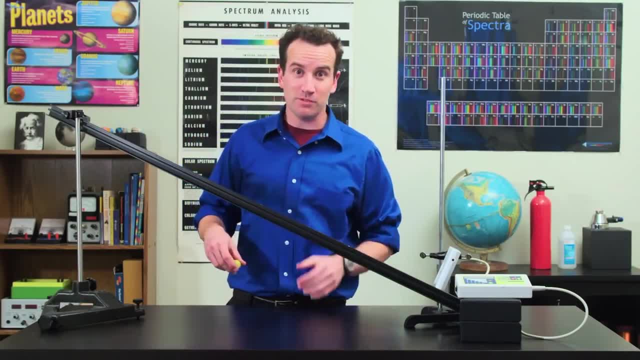 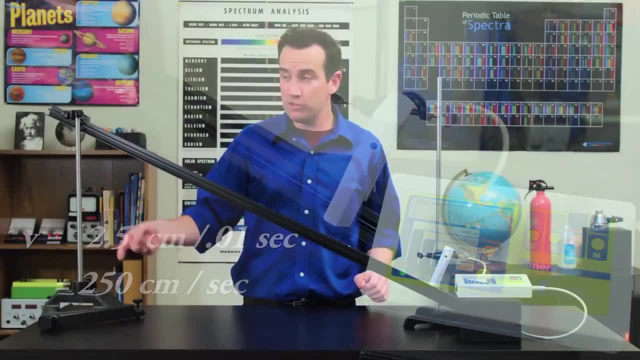 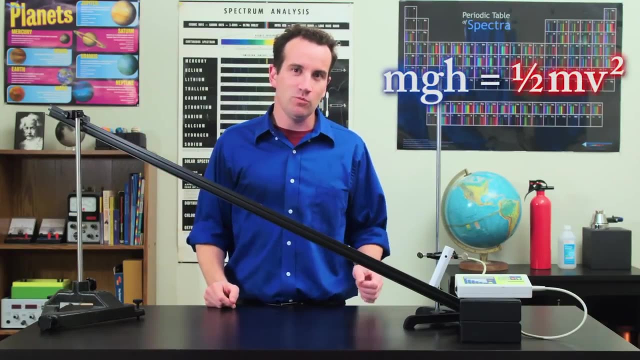 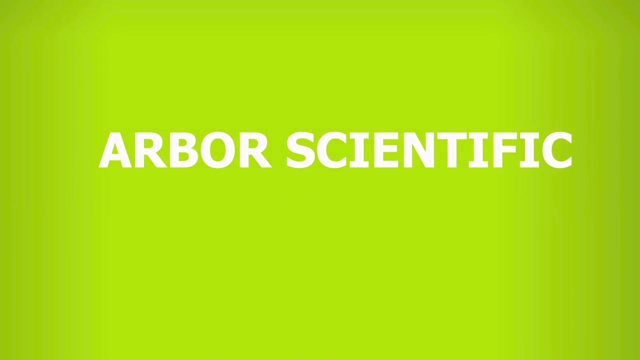 If I want to double the velocity, I have to four times the height There. Four times the height gives you twice the original velocity. The height is increasing with the velocity squared, which is what we expect from potential and kinetic energy. I hope you found this video insightful. 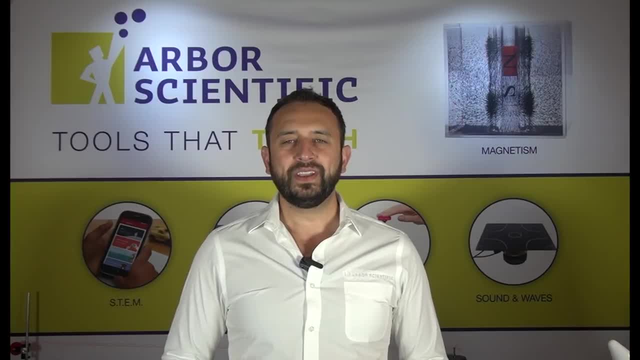 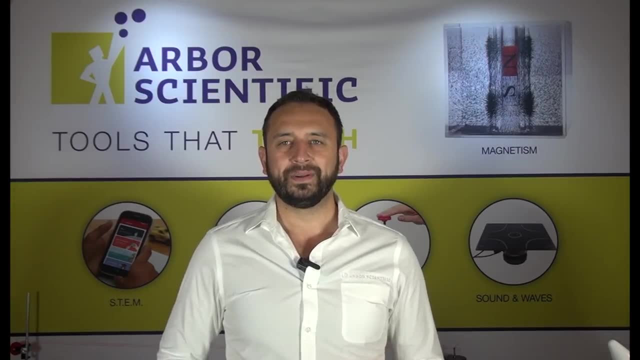 Please leave your thoughts in the comment section below. A new video will be posted every month, So if you enjoyed watching this one, subscribe to our YouTube channel by clicking this link right here And check out some of our other cool videos. If you like watching this one, give us a thumbs up. 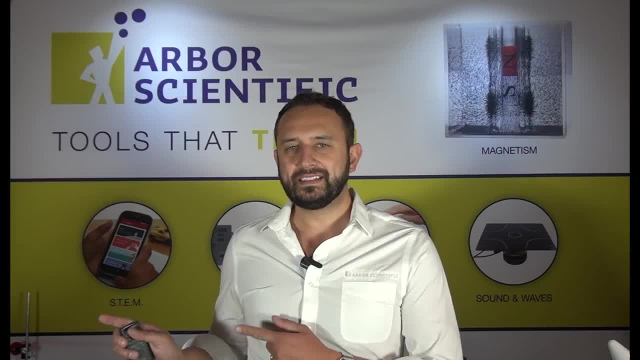 For more information on the products used in this video, click this link right here.